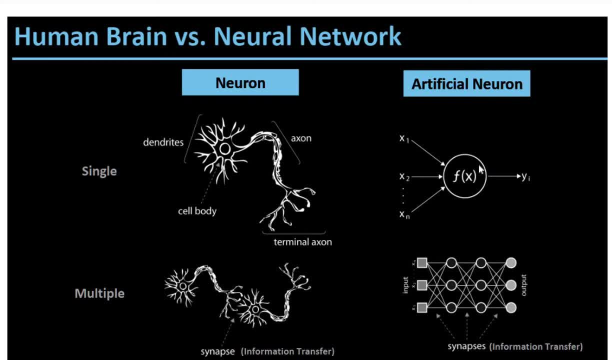 following which the outputs come. Okay, we will study today what those calculations are and what activations are going to be happening. when we look at the Python code, The neuron- this particular case is just a single neuron. that's represented, But right here at the bottom I've written it as multiple, where we have multiple neurons and they have been. 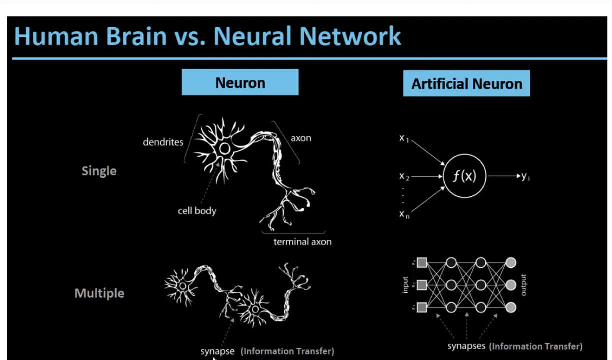 connected using a word called synapse. So what synapse is actually doing is, it is transferring information from one neuron to another neuron, And it is also called the information transfer mechanism system, neural networks. we are going to be using multiple layers, be connected, the key. 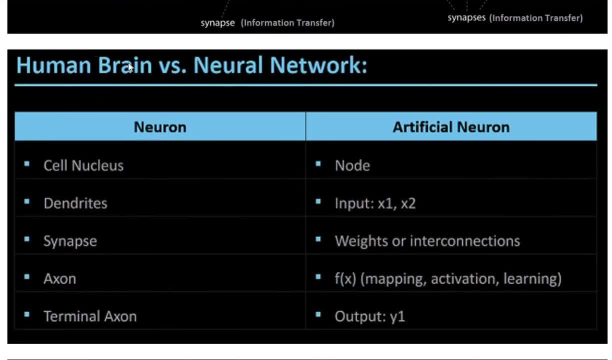 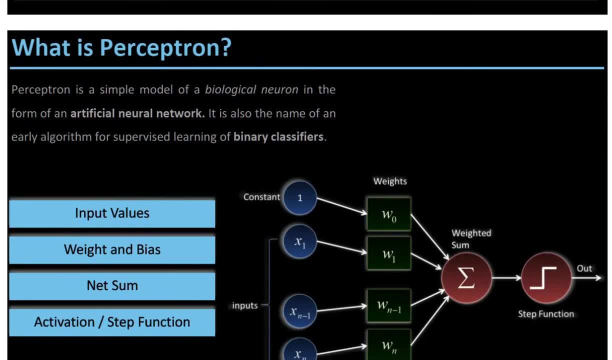 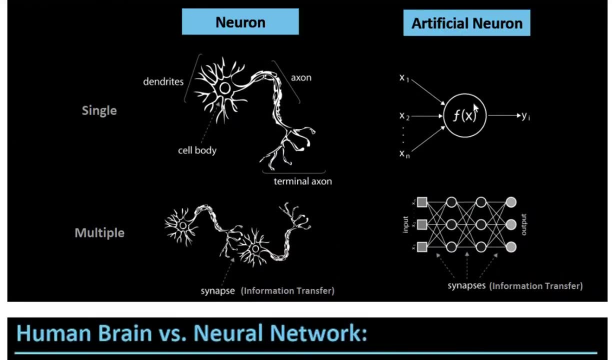 terminologies we have learned between the biological world of human brain and the artificial intelligence in our neural networks. now let's focus our attention on the one single perceptron which we have seen. this, this is just a little elaboration of the same picture I have shown you here. okay, so let us now 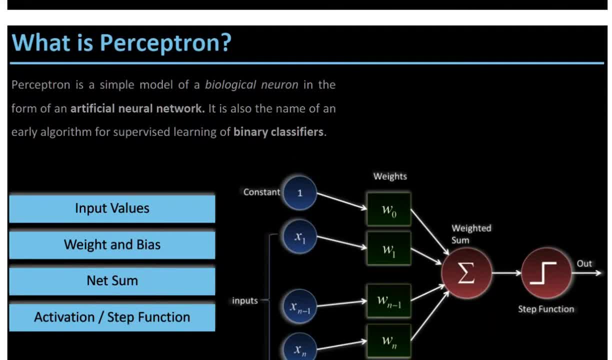 get into the details and understand what is the perceptron and what is the goal of the perceptron algorithm. so perceptron is, as we have seen, a replica of our biological neurons with only one important goal, which is to do classification. okay, that's what it was built for. it has four compone. one is a set of inputs. 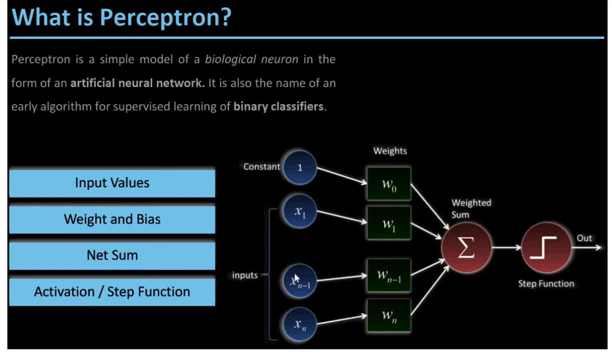 which is X, 1, X, 2, X, 3, ax, n-1 and XN that are actually going into our system. and then we do have the concept of weights and biases. So Whites and Bias, biases, or think of them as coefficients that we have seen in the linear. 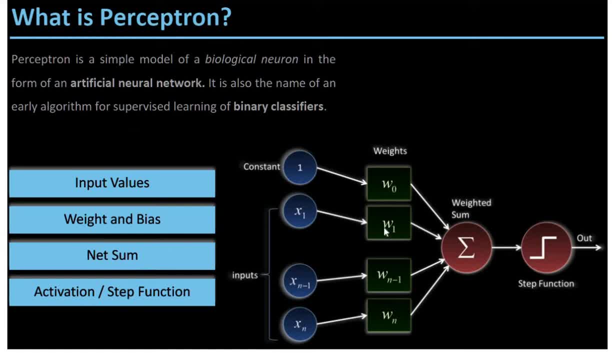 regression or polynomial regression space. so those are weights that are initialized and that are being learned by the system. and then we do have the third component, which is the net sum, which is basically we're putting together all the weights with respect to the inputs and we are weighting them, and 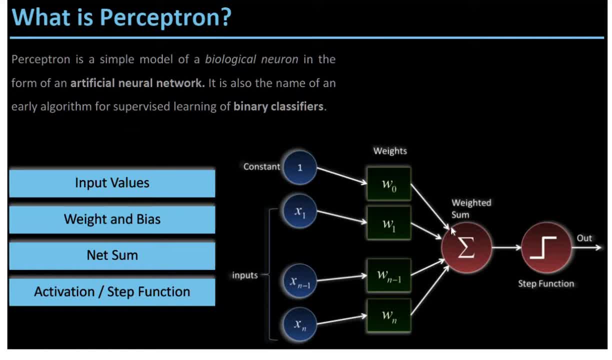 summing them up, which is what this particular summation is standing for, following that, we have an activation slash step function. so, whatever activation we have applied, sometimes we will apply nonlinear activation, which is the majority of the case, and in some cases we will apply linear transformation or linear activation, like the example which we will see today. so 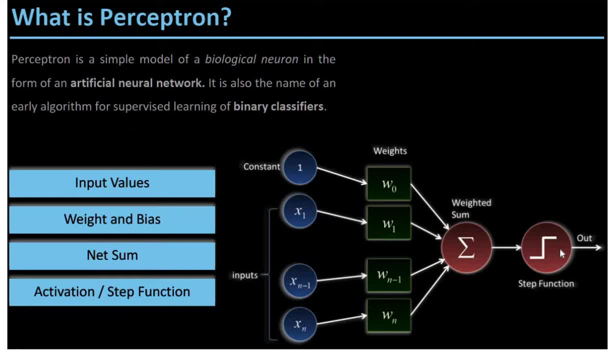 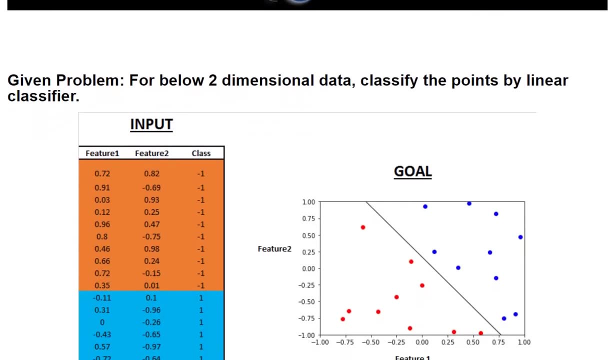 irrespective of what type of activation is applied. we are applying an activation before it goes out. so this is what is the functioning of one single neuron. now we're going to take an example and really walk through each line of code in Python. so let's set the problem up in context. we have been given a problem in hand, the 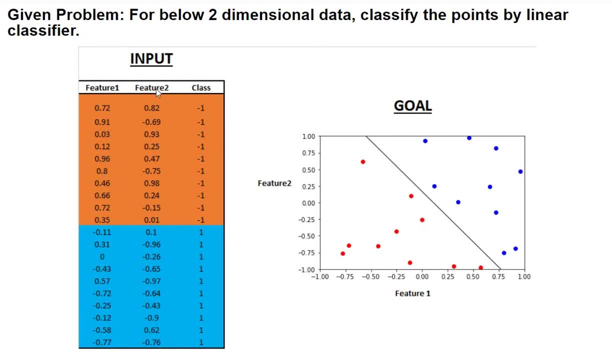 problem is that we have two features, feature 1 and feature 2, and we have the class label for each of the rows. ok, and for our own convenience, what I've done is I have kind of put the red color on the top, or the orange color on the top here, which is referring to all. 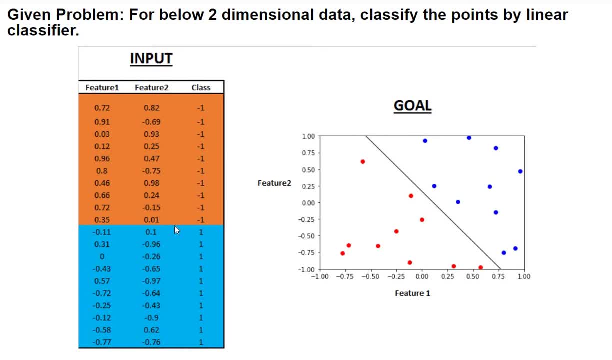 similar classes, which has been labeled as minus one class, and then the blue color on the bottom which is all representing the second class, class number one. so out here in the picture I've shown them, shown the same. so I have one class which is the orange red class, and then the other class which is the blue class. so 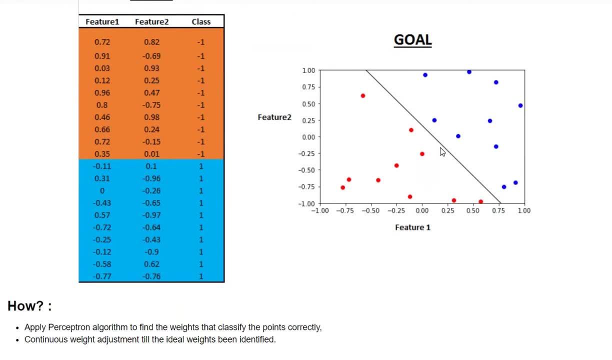 now. we are going to run the perceptron algorithm right now. this black line is our ideal line that we have drawn. now, what are we going to do? we're going to apply the perceptron algorithm to find the weights such that we classify the points correctly. what does that mean? that means the 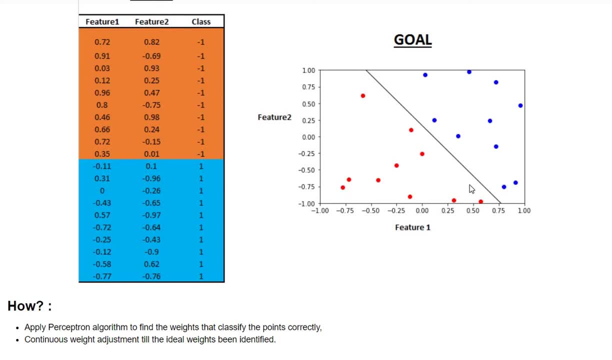 the points are classified correctly. what does that mean? that means the slope of this line, the weights 1 and weights 2 for feature. both features will have to be found, along with any particular bias that might be there. the next thing we're going to also see is that we're going to be continuously. 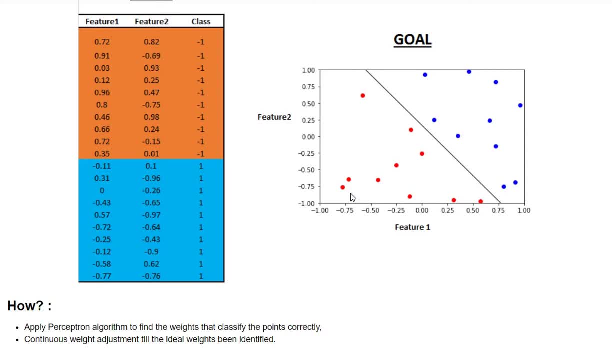 adjusting this weight as part of the algorithm till an ideal line has been found. so that is what the algorithm is going to help us do. to get a better insight of what algorithm is really going to do in step-by-step, before we even see the code, I'm going to show you the output of what we will get from the 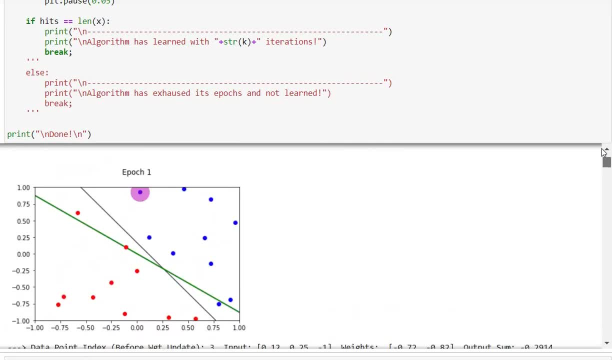 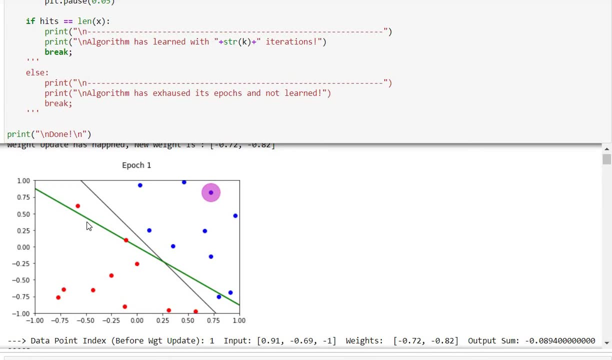 code and then we will understand what's going on. okay, so first, when we start, we are going to basically be having a random line drawn and this random line, we are indicating it in green color. so we have all these data points and this black line I've drawn just to tell you that. 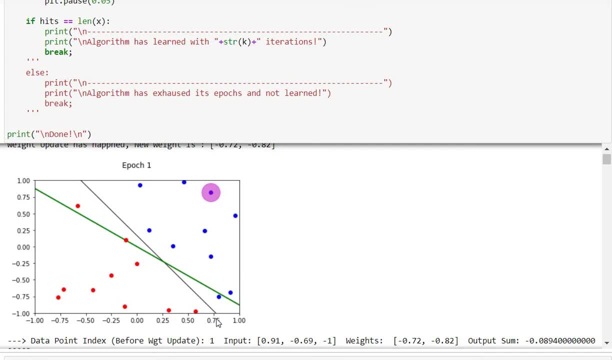 that is the magic line, that is the ideal line. we want to get as close as possible. but we are starting off with a random line, which is the green line. so initially, once we draw this random line, which is based on a random X and y coordinates, what we see is we are seeing that there are many random lines that we can draw. to see if we draw them specifically. 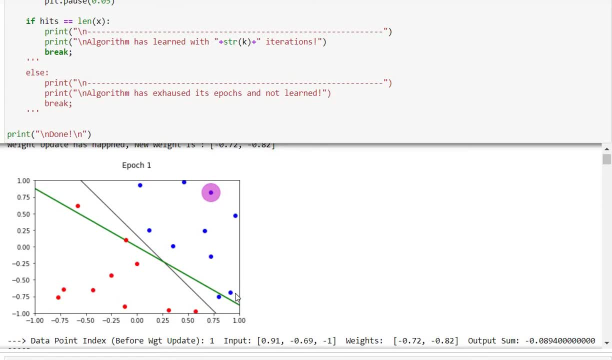 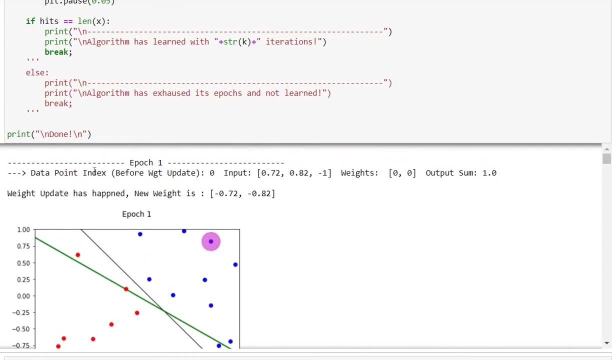 what we see is we are seeing that there are errors, we are seeing that it is not perfectly classified. It has multiple errors for red point and possibly one error for blue point. So those things are all going to be marked. So it is going to fundamentally learn the steps to say: look first, initially my weights. 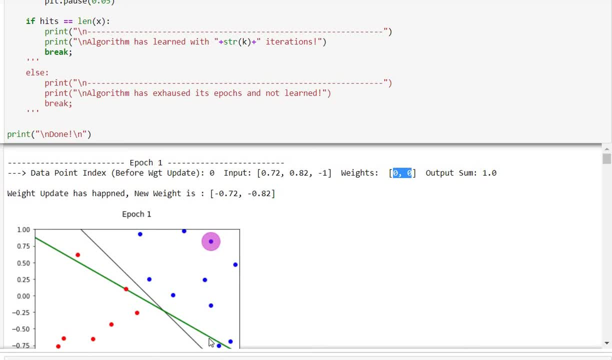 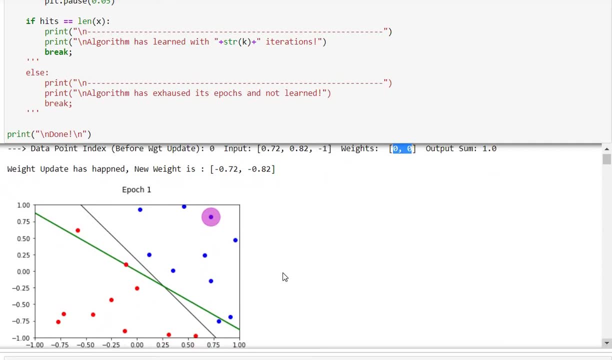 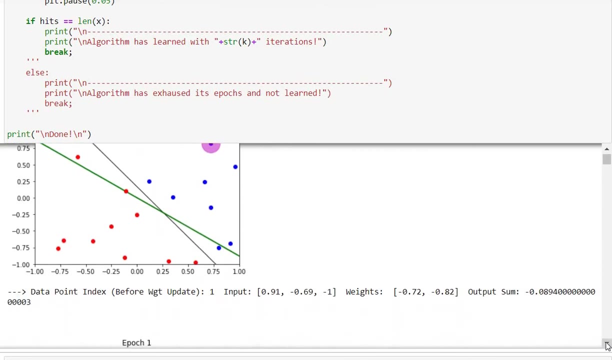 are going to be zero And I've drawn a random line After that, after drawing the random line, I have to update the weights in such a way that my errors, these red errors, are minimized And even though it's just one point, a blue error is minimized. So let us see what. 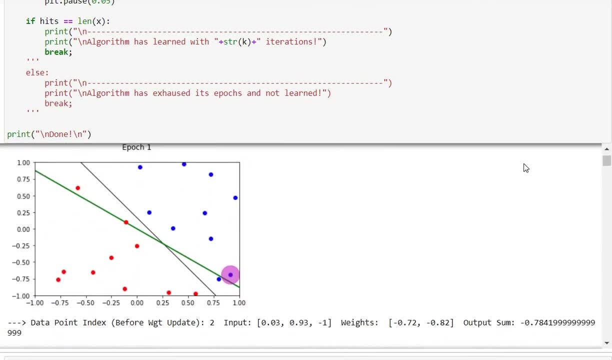 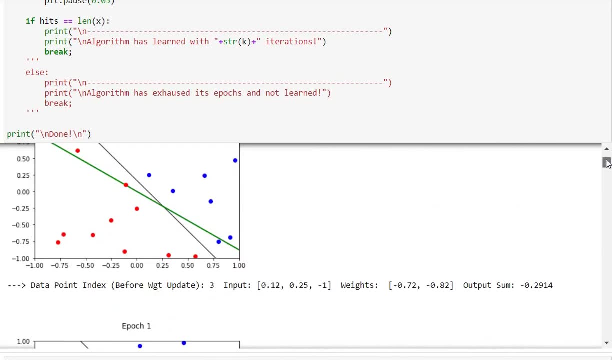 happens in the next epoch. These are all happening for each data point, So I'm going to go to the epoch number two to show you how this line is starting to shift. All right, so let's come back up here before I go to epoch number two. And this is for each data point. So first, 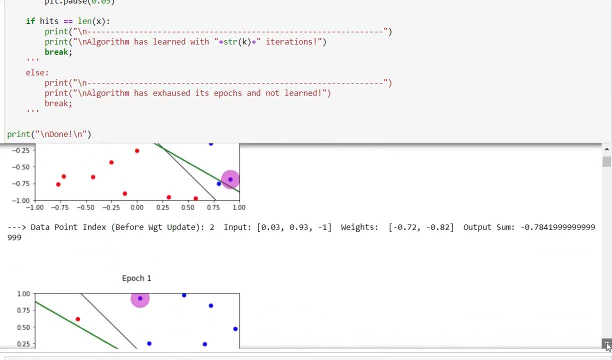 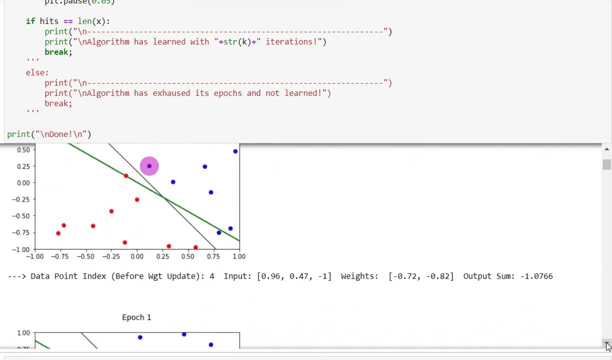 data point comes in. Second data point comes in. Second data point comes in. Third data point, The third data point. again, the line is shifting slightly, if you might see. In the fourth data point there are actually no errors right now, Till this point there. 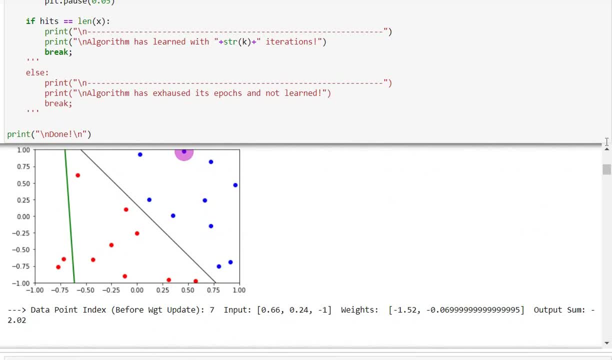 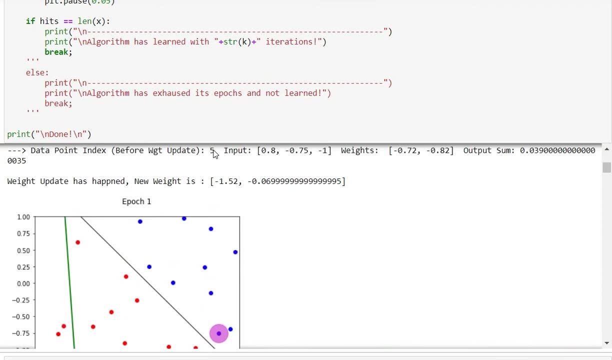 is no errors, So the line is really not shifting that much. But the moment we came at this point, at this point where we have a data point index, data point number five, we can see the line has shifted significantly. That was the new green line. 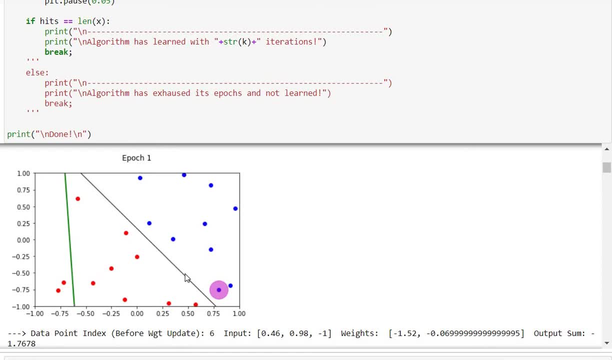 The green line is drawn like this, even though our ideal line was like this. So now, if we evaluate what the errors are, we probably have drawn a really poor line of segregation. The errors are possibly a lot more, So we'll continue iterating again to try and minimize. 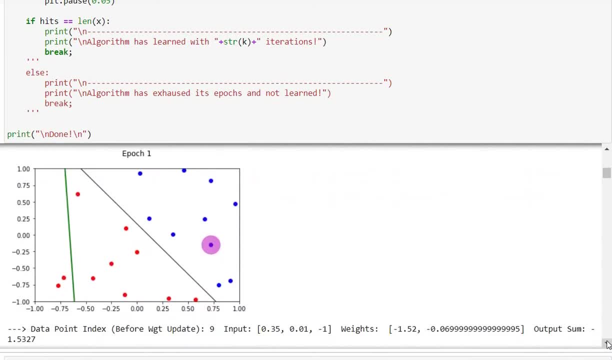 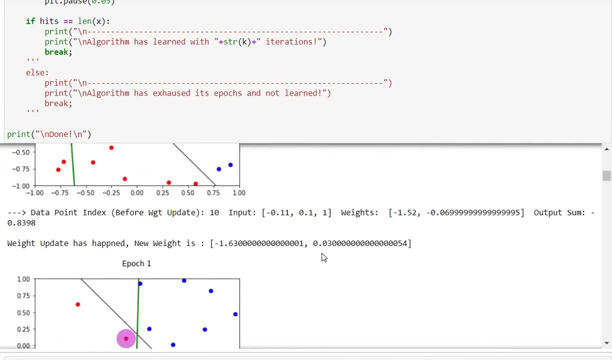 that error as we go through each data point within the epoch. So let us see where else we have a major change. And again, at this point, of the data point number 10, because that is the last data point- we have 10 data points. 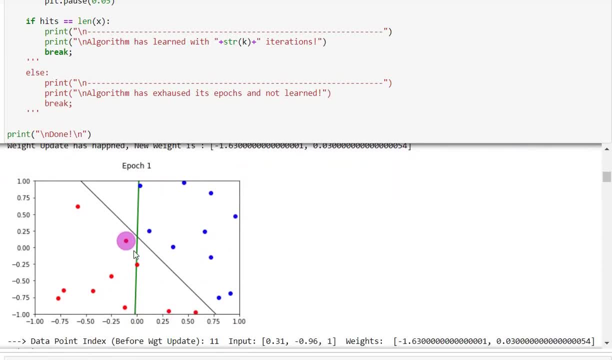 We are starting to see the line has shifted again, more to the right this time, And this time it again has two errors, and this is a point that is right on the line, But the blue points, if you observe, have actually been correctly identified. There are no errors. 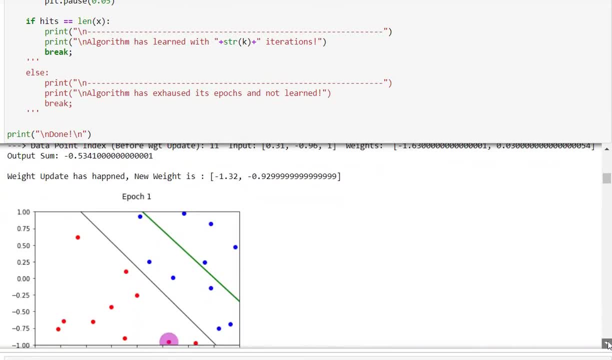 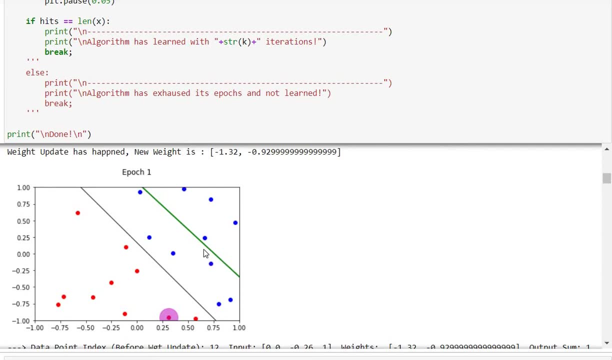 in the blue points. So this goes on this concept of it moving the line to try and find an ideal split in such a way that the errors are zero or at least minimum for the given epoch. So that's the important message I want you guys to take. 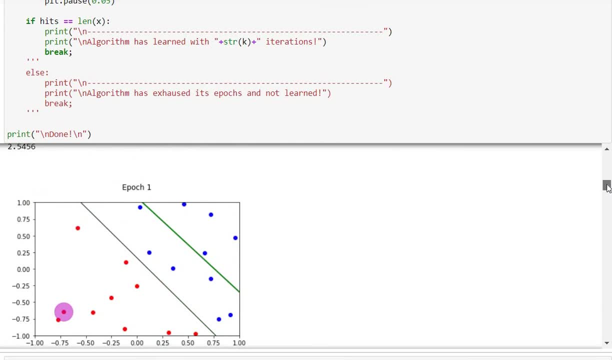 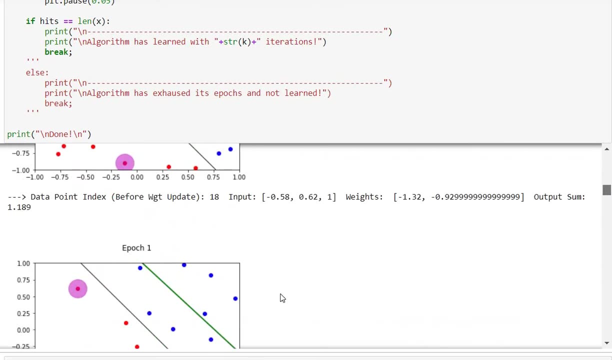 And, as we will see, as it goes through more and more epochs. so we are still in the first epoch, which means we are putting through all data points, one data point after another. in our example, we are putting that through And I'm highlighting which is the data point. 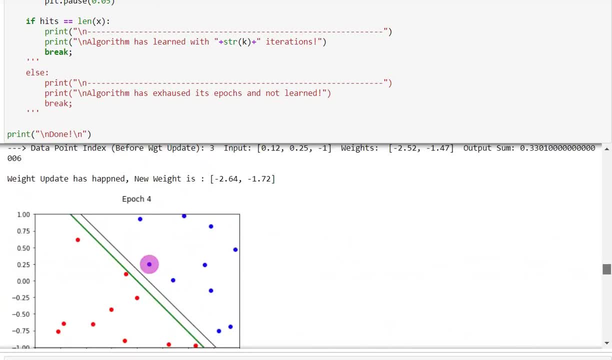 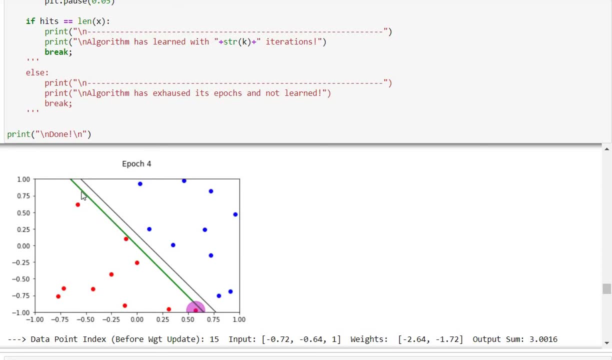 we are currently processing through these colors. So let's go down, let's go down, let us see what it really has learned. So, when it came from epoch one to epoch four, there has already been an improvement, a significant improvement, where it has already drawn the green line. Much, much similar. 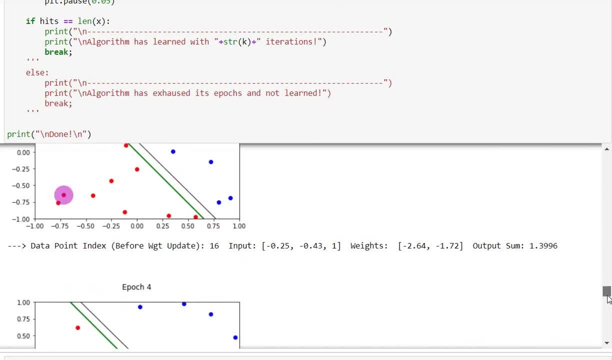 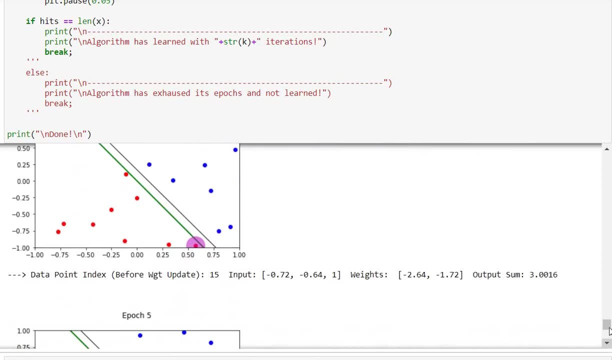 Much, much similar and parallel to the black line, which was our ideal line. All right, let's come down further, Further down. I'm going into epoch number five. I'm seeing if there is any improvement in epoch number five. Yes, there has been some improvements. 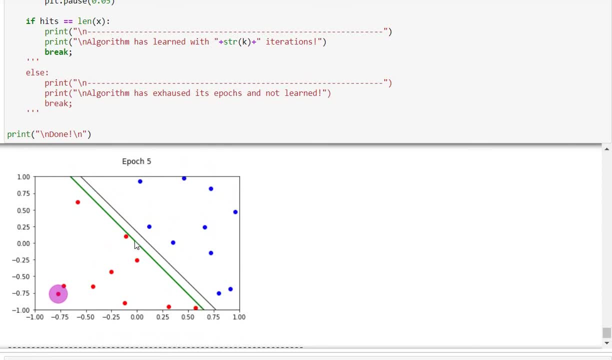 And then finally, once it's finished, epoch number five, what we can see is it has perfectly classified my red points from my blue points and it has drawn the line. It is not exactly drawn on the ideal line that we had benchmarked, which is the black line, but it found a solution. 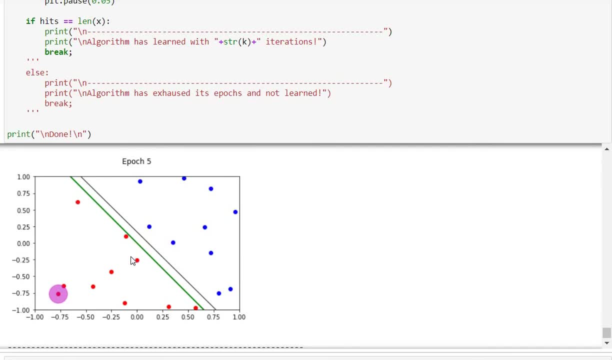 which satisfies the main constraint, which is the red points should be separated from the blue points. So now that we understood what the algorithm has actually done iteratively, let us now go and take a look at the code to really see how we did it. So it's really simple code. So first let's get our imports in place. 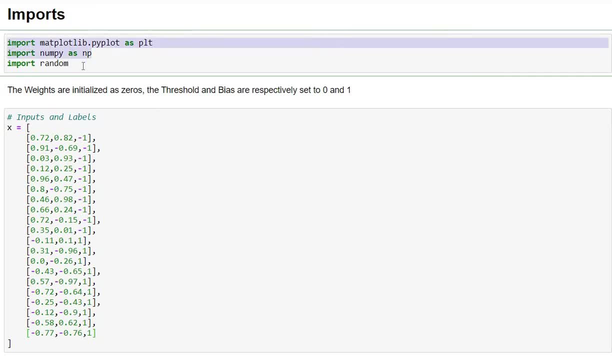 So what are we importing? We are importing matplotlib, we are getting numpy and we are getting random. This random is helpful for us to get some random numbers. Next, we are putting in our inputs. So this is the inputs that have been given to us. 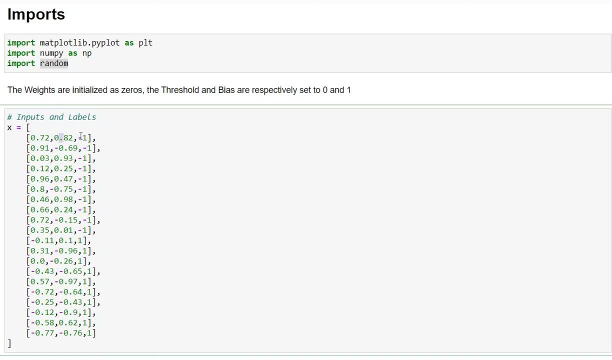 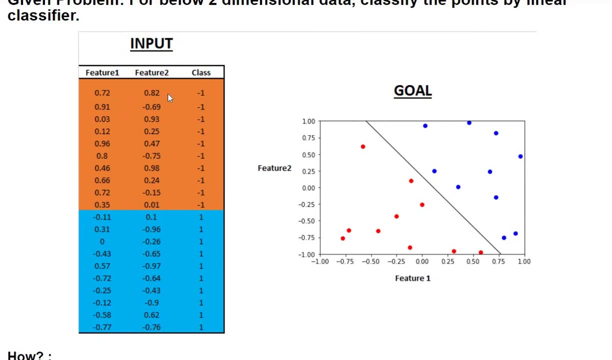 This is given to us, like these are the feature one, feature two and the label. So this is something I've shown you earlier as how I put it in the grid here in multiple colors, but that same values is what we are now getting as inputs, both as an array and also we are. 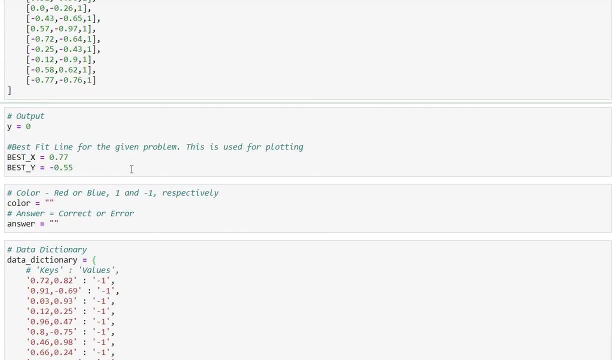 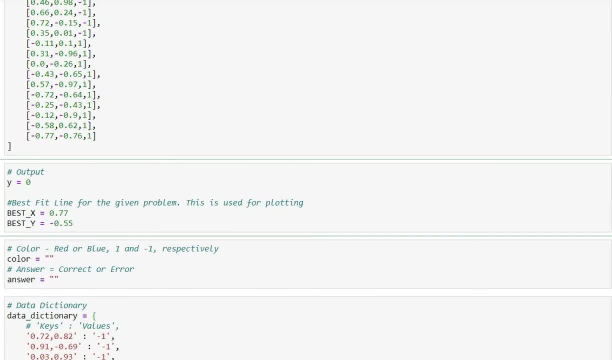 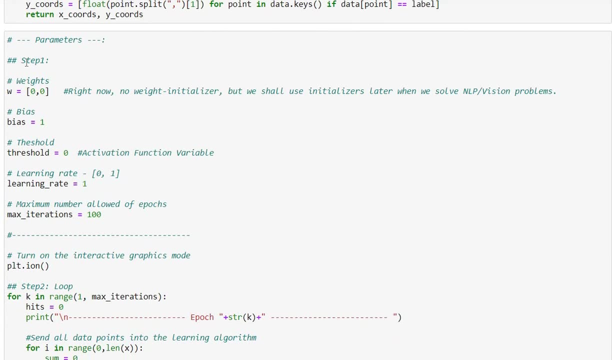 we knew the answer for this problem. therefore, we were able to do this. All right, so now we'll go down and let us take a look at the main function. So the main function has got three steps. Step number one is we are going to go and initialize the. 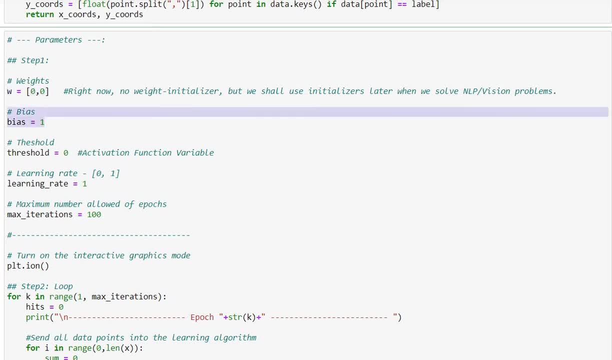 weights. Initially we are initializing it to 0,, 0. Then the bias again is not initialized to 0, but its bias is initialized to 1.. Then we are setting up a threshold which is nothing but our activation functions, one of the variables we use in the activation function, And then 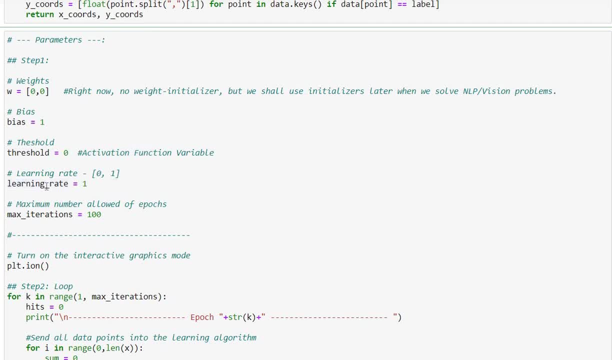 we are setting up our bump parameter to be 1, which is we are calling it the learning rate. This measures how much are we going to be moving the coefficients as we search for a solution, And then the maximum number of epochs we want to try. that is in this. 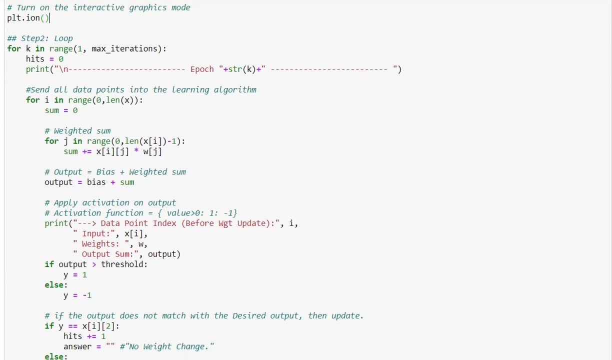 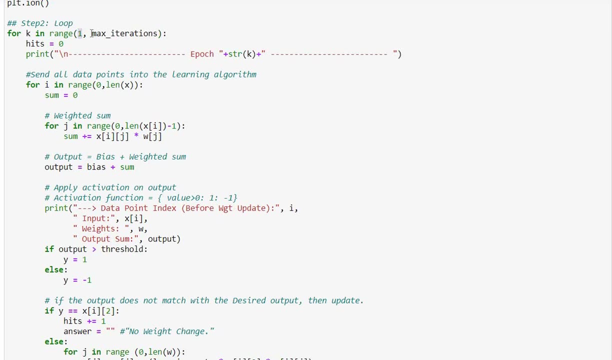 variable. Following that, we are basically setting up a graphics mode and then we are going into the step two. Step two is looping in for each of the epochs. So we have set from 1 to maximum number of epochs, We are going to be iterating And within that, for 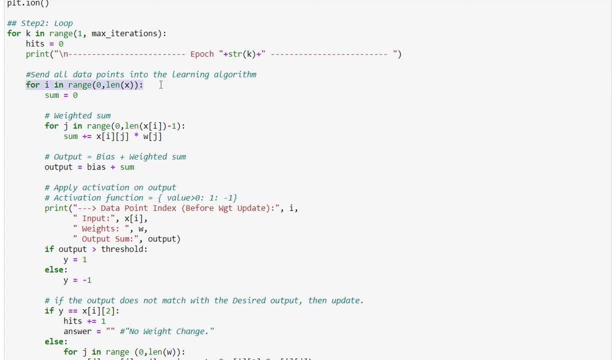 each epoch, we will be iterating across each data point in our overall input space. So that's what this i is going to be carrying. So this is the second for loop for i in range of 0, ln of x. Following that, we are doing a very important calculation here, which is: 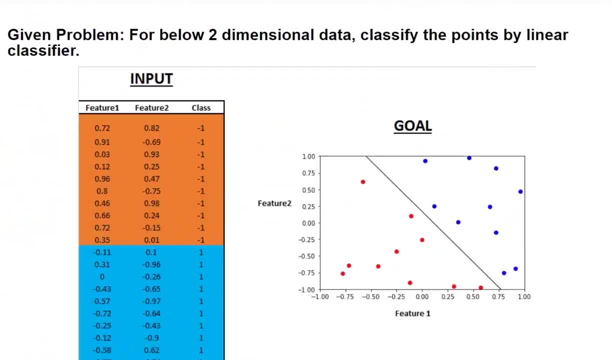 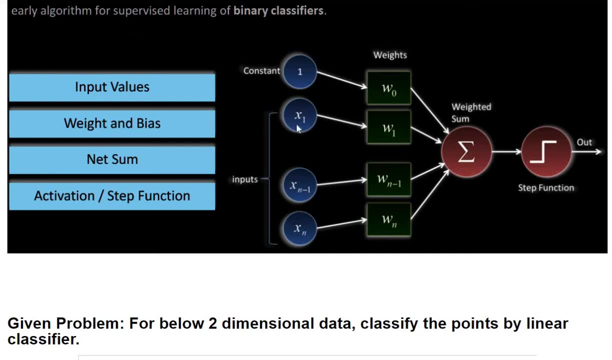 the weighted sum. So you would have seen it out here I explained that there is something called as a weighted sum, which is nothing but taking in the weights, taking in the corresponding inputs, multiplying them and then summing all of those. 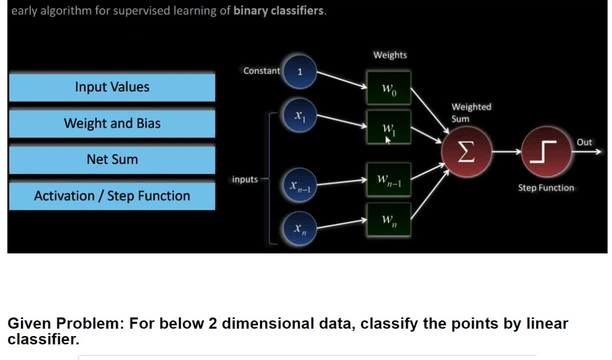 So, fundamentally, you are taking x1 into w1, plus x2 into w2, xn-1 into wn-1, plus xn into wn. That is what we are doing. That is our weighted sum In the code. all we are doing. 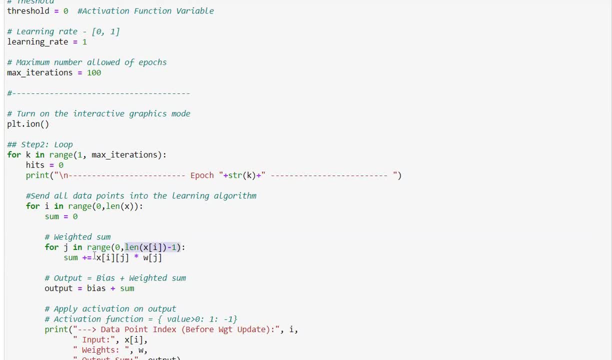 is, we are going in for each of the input variables we have, We are multiplying it with the corresponding coefficient, which is in our w variable. x is my input variable, And then I am just adding them all up. So this would give me my weighted sum. 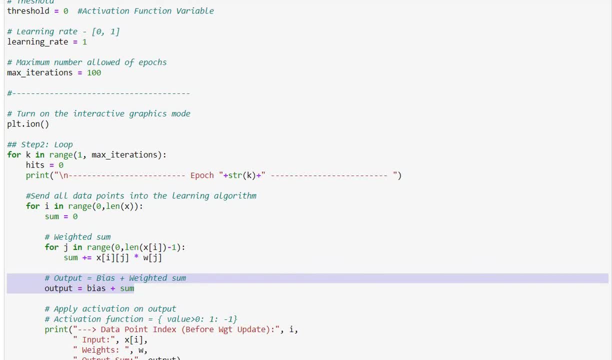 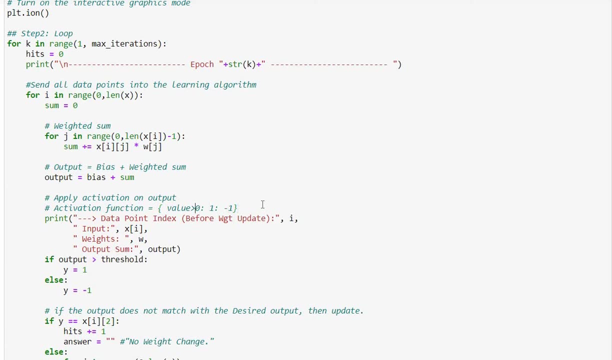 I would basically have a bias, so I would be adding the bias to the weighted sum, following which I apply my activation function. So in this particular case, the activation function is really simple. All I have said is: if this value, this is the output. if it is greater, 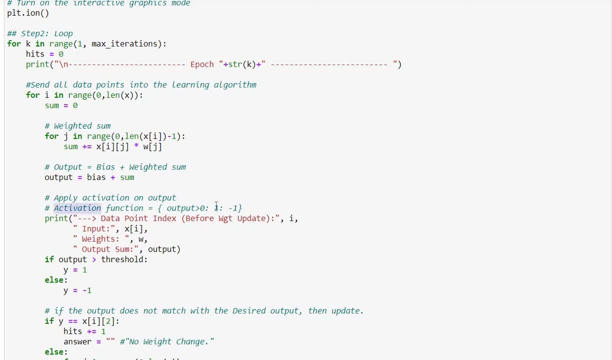 than 0,, then my return value from the activation is 1.. And if it is less than 0, then my return value out of this activation is minus 1.. So once I do that, then I have my values going out. My output has been transformed using an activation function, which is what we have. 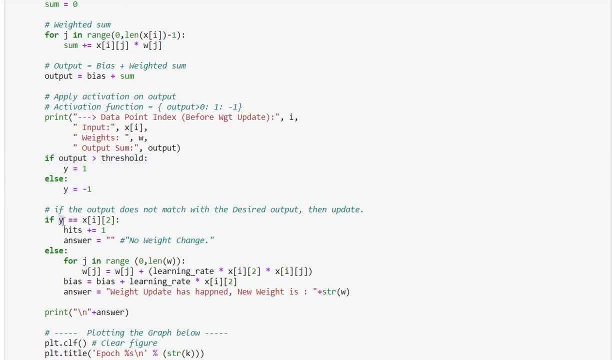 here I am going to do a new variable, which is the y variable. So for the y variable, now we are going to be checking whether it matches with my class variable or not. If it matches to my class, then nice and fine. very good, My output is useful. If it is not matching, 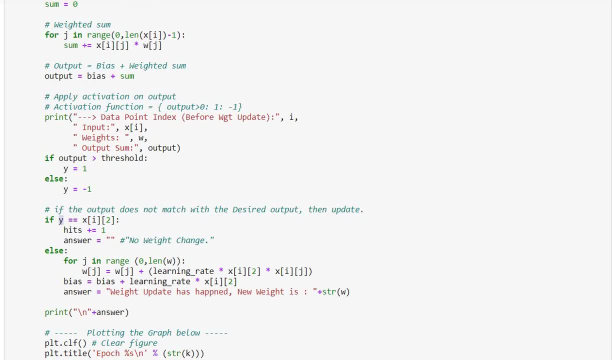 with my class. when I say class, whether it is minus 1 or plus 1, then I have to update the weight. So what this literally meant is, if my output for the given input value, if my output that I calculated- is as expected, I will not do anything. But if it is not as 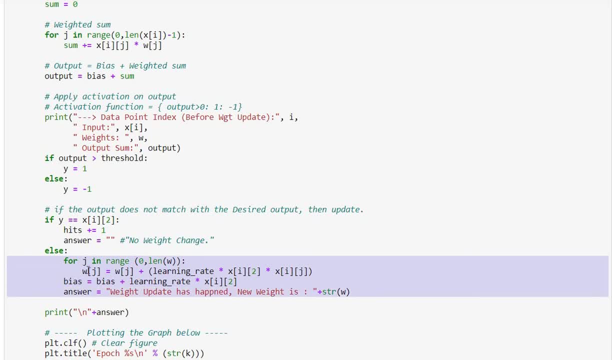 expected the proposed method was and the advantage of the ways, Then use the algorithm to set up some ال. If i mean take all data colored data今 저는 tallcat, Then I would have to update my weights. So I am updating my weight here using my learning. 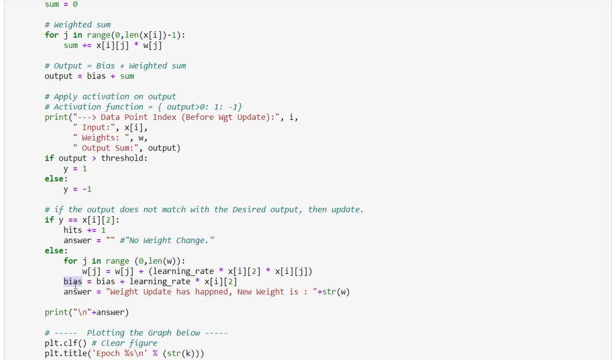 rate as my bump value. Following that, I am actually finishing that up for each coefficient of the weight. So I have 2 coefficients in weights- weight 1, weight 2, because I have 2 inputs, feature 1 and feature 2.. 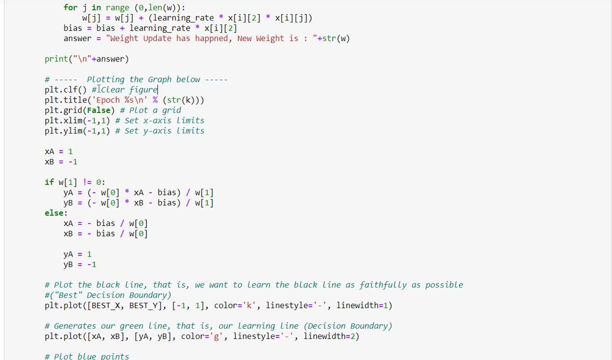 I am also updating the Bias, which is only 4 ones Following that. so that is really the algorithm, That is really the core of the algorithm. Following that, I have done some code, basically to do plotting. What I have done so far is I: 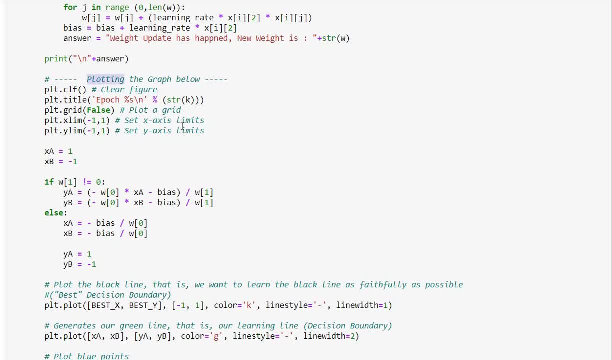 have done a sloppy production, but which means, if I already have some hard code that has something, I've done the plot work so that we can highlight certain data points and also understand how close is this green line. But let us now run this and see what happens.